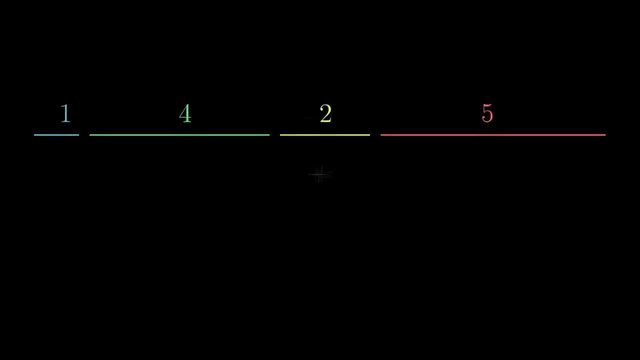 Usually with averages, we think of a finite number of variables where we can add them all up and divide that sum by how many there are. But there's infinitely many values of sine, of x, between zero and pi, and it's not like. 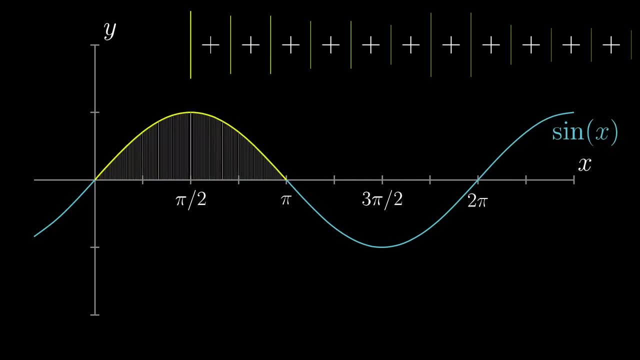 we can just add up all of those numbers and divide by infinity. This sensation actually comes up a lot in math and it's worth remembering Where we this vague sense that what you want to do is add together infinitely many values associated with a continuum, even though that doesn't really make sense, And almost always when 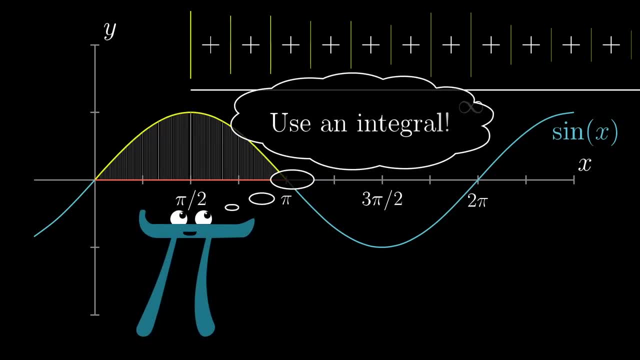 you get that sense. the key is going to be to use an integral somehow And to think through exactly how a good first step is usually to just approximate your situation with some kind of finite sum. In this case, imagine sampling a finite number of points evenly. 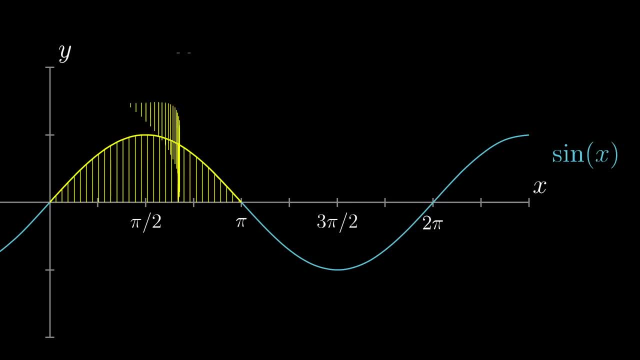 spaced along this range. Since it's a finite sample, you can find the average by just adding up all of the heights sine of x at each one of these and then dividing that sum by the number of points that you sampled right. 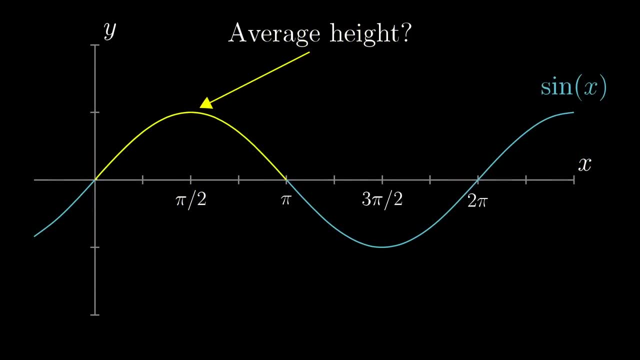 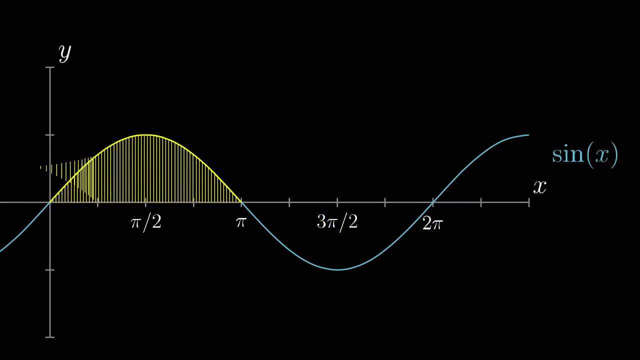 And presumably if the idea of an average height among all infinitely many points is going to make any sense at all, the more points we sample, which would involve adding up more and more heights, the closer the average of that sample should be to the actual average. 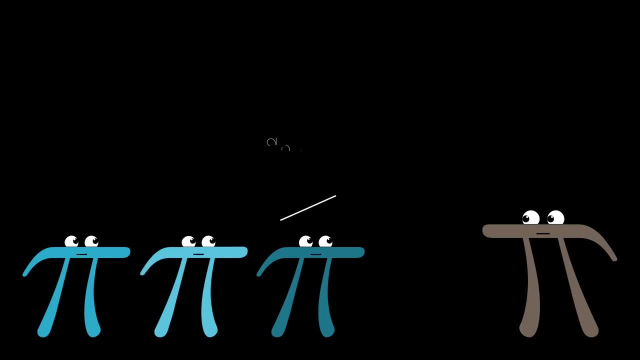 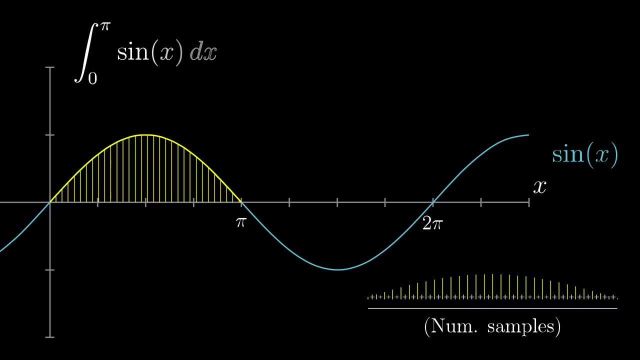 of the continuous variable, And this should feel at least somewhat related to taking an integral of sine of x between zero and pi, even if it might not be exactly clear how the two ideas match up. For that integral, remember you also think of a sample of inputs on this continuum. but instead of 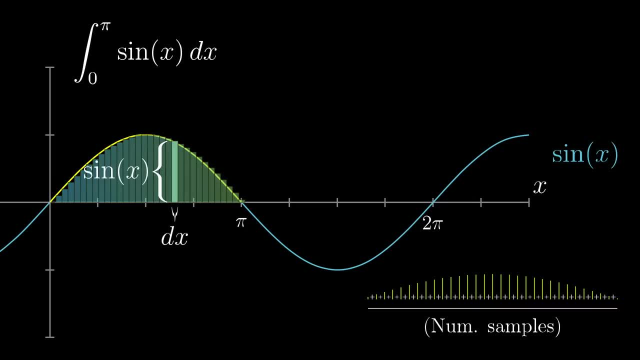 adding the height sine of x at each one and dividing by how many there are, you add up sine of x times dx, where dx is the spacing between the samples. That is, you're adding up little areas, not heights. 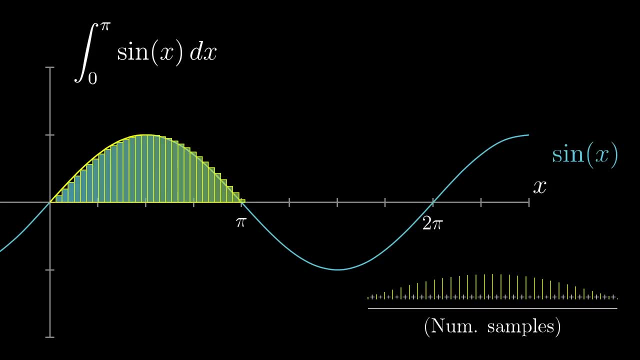 And technically the integral is not quite this sum. it's whatever that sum approaches, as dx approaches zero. But it is actually quite helpful to reason with respect to one of these finite iterations where we're looking at a concrete size for dx and some specific 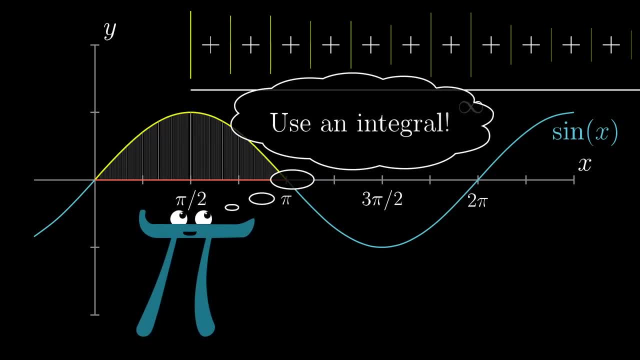 when you get that sense, the key is going to be to use an integral somehow And to think through exactly how a good first step is usually to just approximate your situation with some kind of finite sum. In this case, imagine sampling a finite number of points. 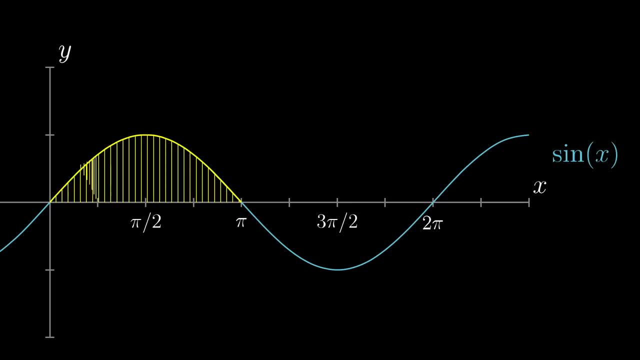 evenly spaced along this range. Since it's a finite sample, you can find the average by just adding up all of the heights sine of x at each one of these and then dividing that sum by the number of points that you sampled right. 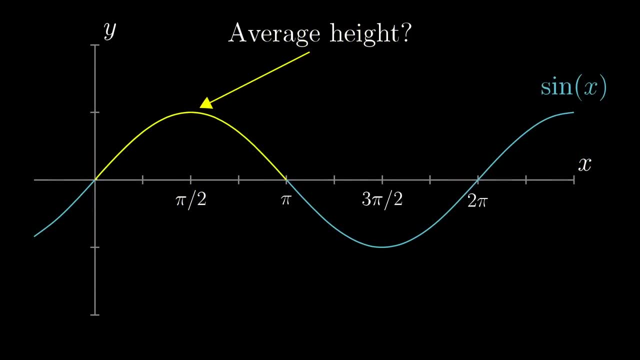 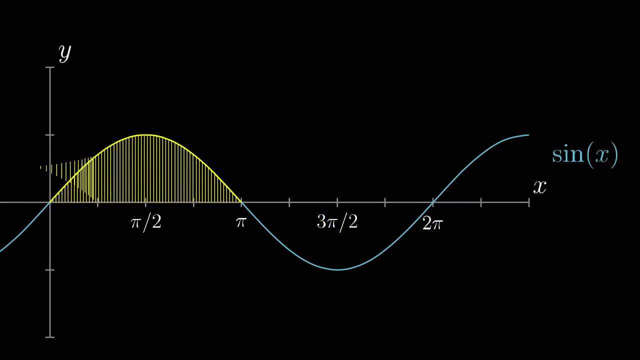 And presumably if the idea of an average height among all infinitely many points is going to make any sense at all, the more points we sample, which would involve adding up more and more heights, the closer the average of that sample should be to the actual average. 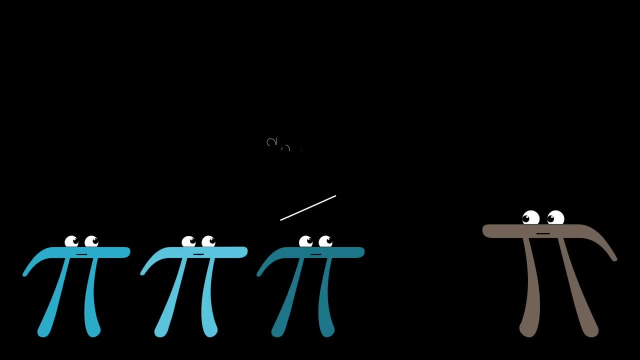 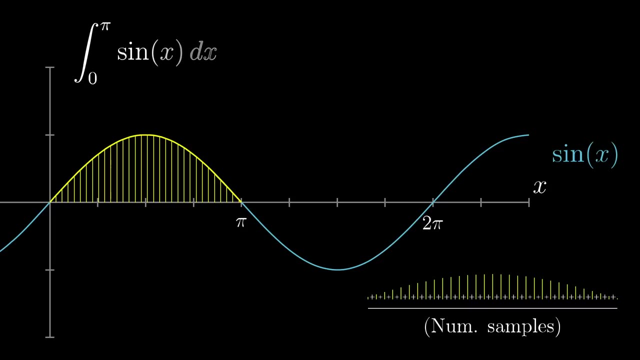 of the continuum, And this should feel at least somewhat related to taking an integral of sine of x between zero and pi, even if it might not be exactly clear how the two ideas match up For that integral. remember, you also think of a sample of inputs on this continuum, but instead of 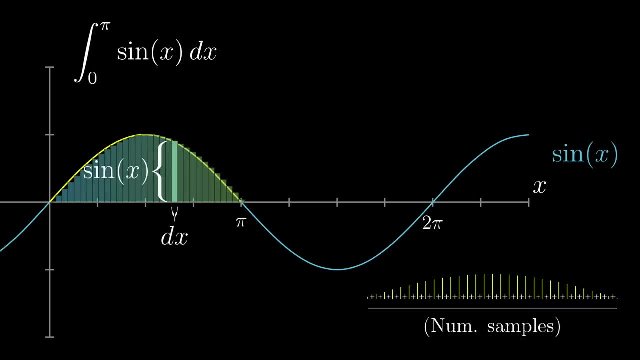 adding the height sine of x at each one and dividing by how many there are, you add up sine of x times dx, where dx is the spacing between the samples. That is, you're adding up little areas, not heights. 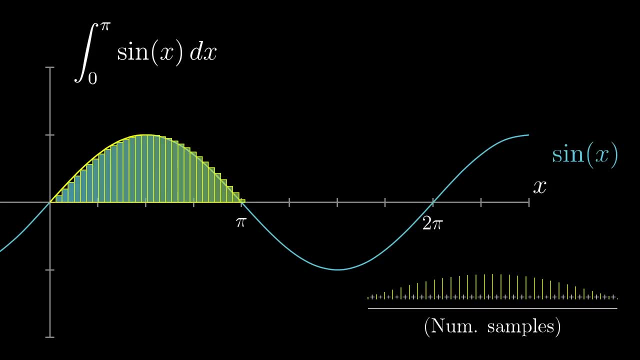 And technically the integral is not quite this sum. it's whatever that sum approaches, as dx approaches zero. But it is actually quite helpful to reason with respect to one of these finite iterations where we're looking at a concrete size for dx and some specific 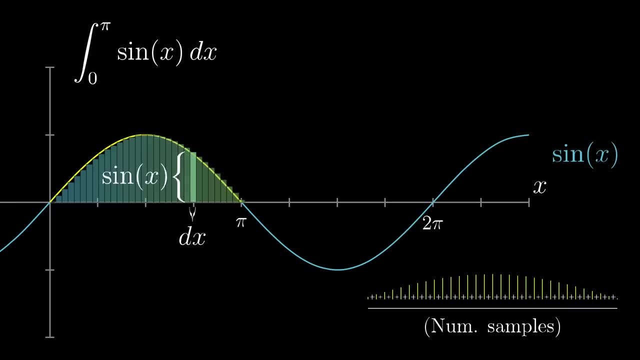 number of rectangles. So what you want to do here is reframe this expression for the average, this sum of the heights divided by the number of sampled points in terms of dx. So what you want to do here is reframe this expression for the average, this sum of the. 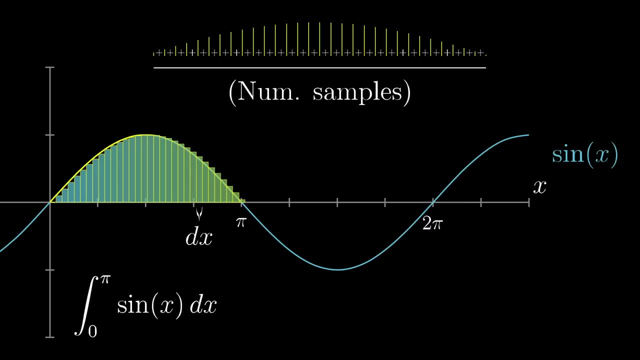 heights divided by the number of sampled points in terms of dx at each one of these points. And that's what we're going to do here. That's what we're going to do here And now, if I tell you that the spacing between these points is, say, 0.1, and you know that, 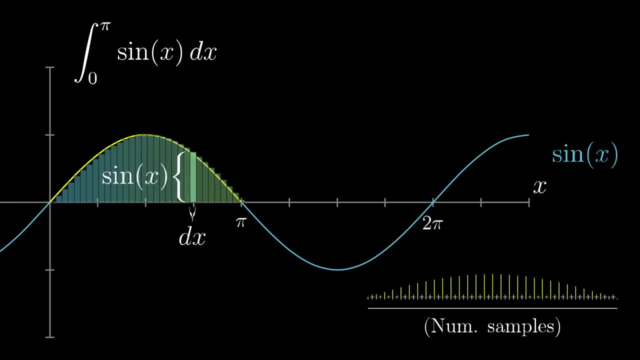 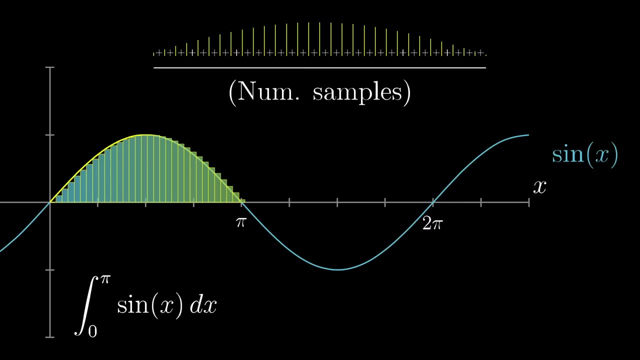 number of rectangles. So what you want to do here is reframe this expression for the average, this sum of the heights divided by the number of sampled points in terms of dx. So what we're going to do here is reframe this expression for the average, this sum of the heights divided by the number of sampled points in terms of dx and sine of x. 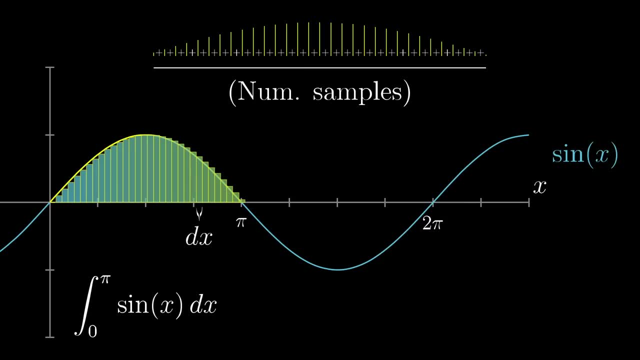 And if I tell you that the spacing between these points is, say, 0.1, and you know they range from 0 to pi, can you tell me how many there are? Well, you can take the length of that interval, pi, and divide it by the length of the space. 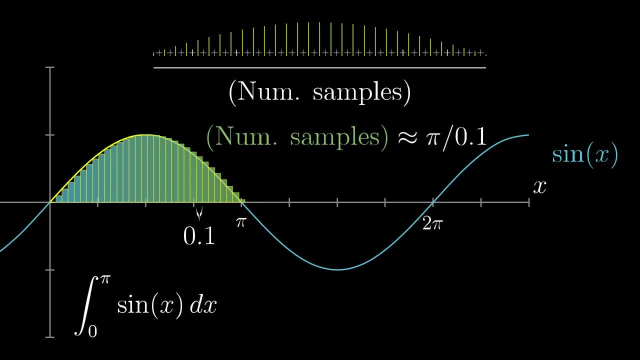 between each sample. If it doesn't go in perfectly evenly, you would have to round down to the nearest integer, But as an approximation this is quite simple. So if we write that spacing between samples as dx, the number of samples is pi divided. 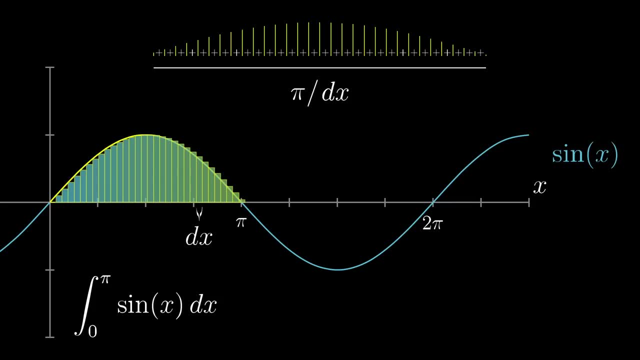 by dx And when we substitute that into our expression, you can rearrange it, putting that dx up top and distributing it into the sum. But think about what it means to distribute that dx up top. It means that the terms you're adding up will look like sine of x times dx for the various 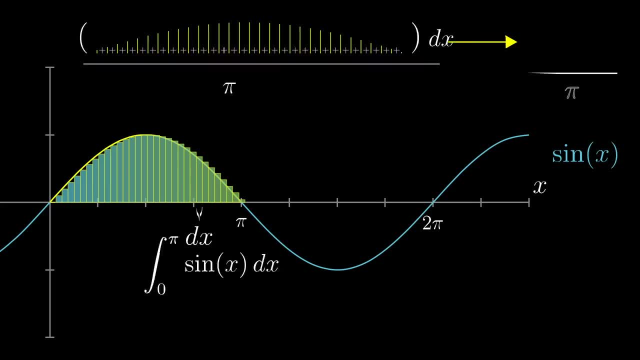 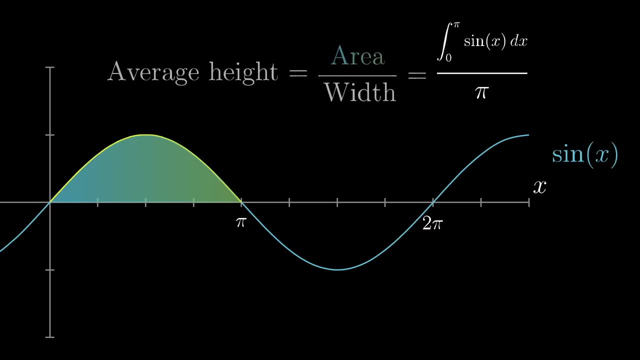 inputs x that you're sampling So that numerator looks exactly like an integral expression. And so for larger and larger samples of points, this average will approach the actual integral of sine of x between 0 and pi all divided by the length of that interval, pi. 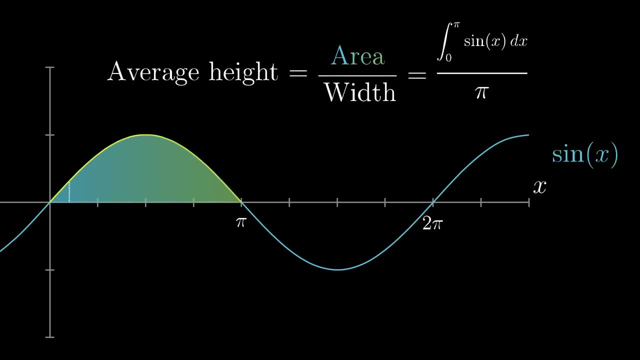 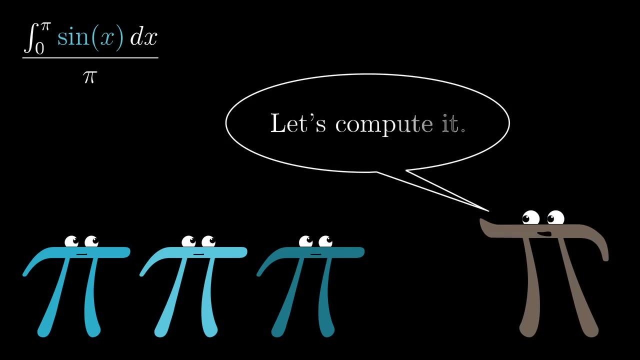 In other words, the average height of this graph is this area divided by its width. On an intuitive level, and just thinking in terms of units, that feels pretty reasonable, doesn't it? So, with this expression in hand, let's actually solve it. 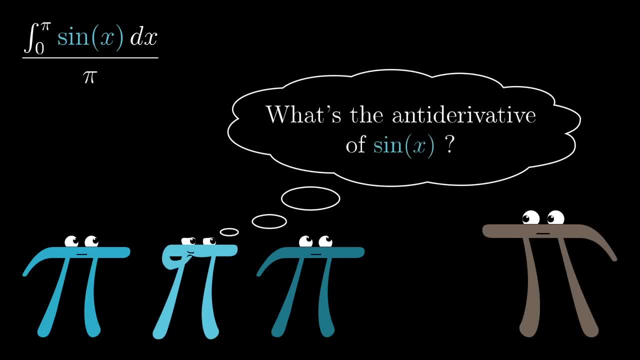 As we saw last video, to compute an integral you need to find an antiderivative of the function inside the integral, some other function whose derivative is sine of x. And if you're comfortable with derivatives of trig functions, you know that the derivative 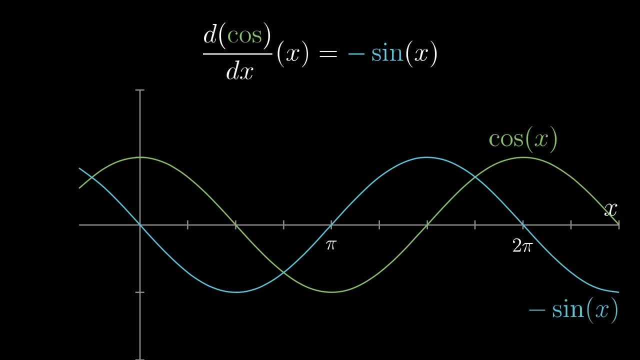 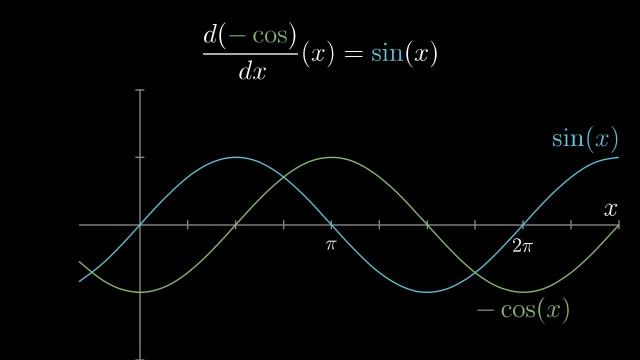 of cosine is negative sine. So if you just negate that negative cosine is the function, we want, The antiderivative of sine. And to gut check yourself on that, look at this graph of negative cosine At 0, the slope is 0.. 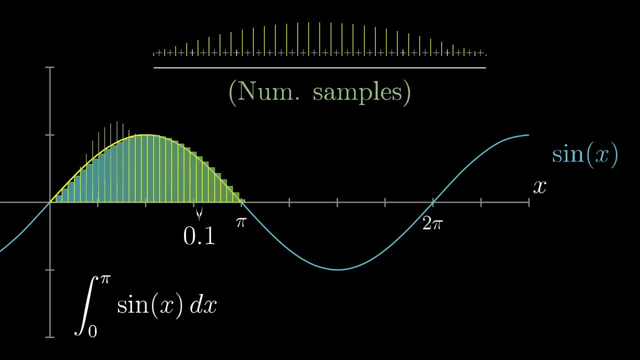 they range from 0 to pi. can you tell me how many there are? Well, you can take the length of that interval, pi, and divide it by the length of the space between each sample. If it doesn't go in perfectly evenly, you would have to round down to the nearest integer. 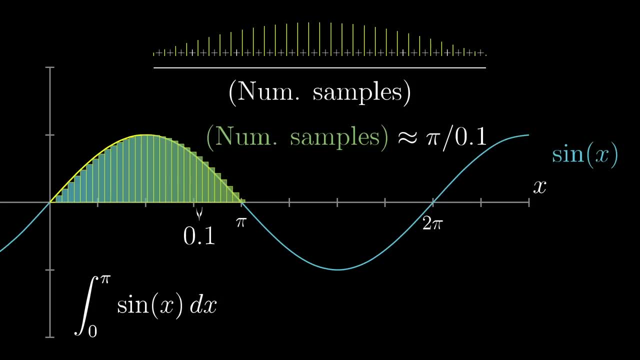 but as an approximation This is completely fine. So if we write that spacing between samples as dx, the number of samples is pi divided by dx, And when we substitute that into our expression up here, you can rearrange it, putting that dx up top and distributing it into the sum. 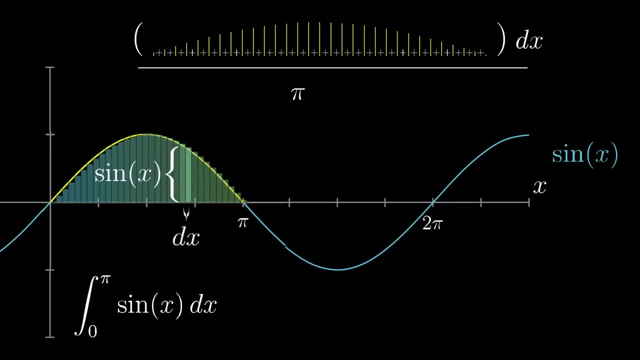 But think about what it means to distribute that dx up top. It means that the terms you're adding up will look like sine of x times dx for the various inputs x that you're adding up, So that numerator looks exactly like an integral expression. 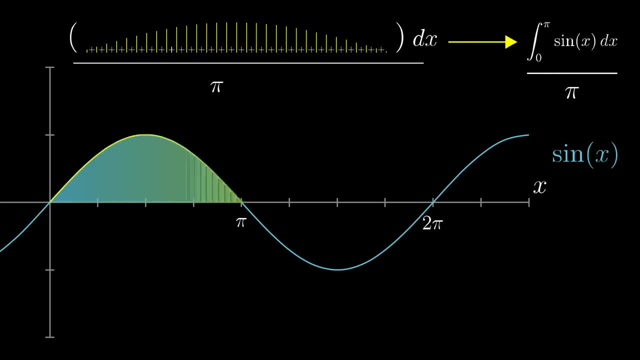 And so for larger and larger samples of points. this average will approach the actual integral of sine of x between 0 and pi, all divided by the length of that interval. pi, In other words, the average height of this graph, is this area divided by its width. 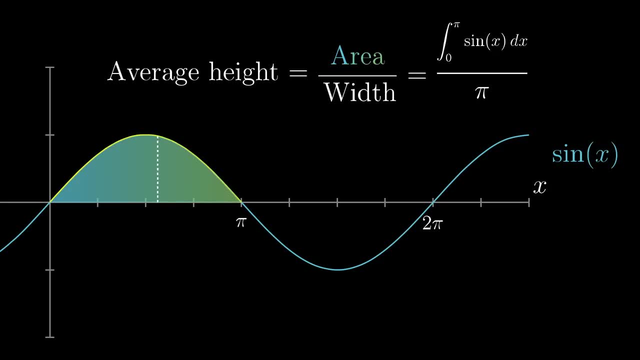 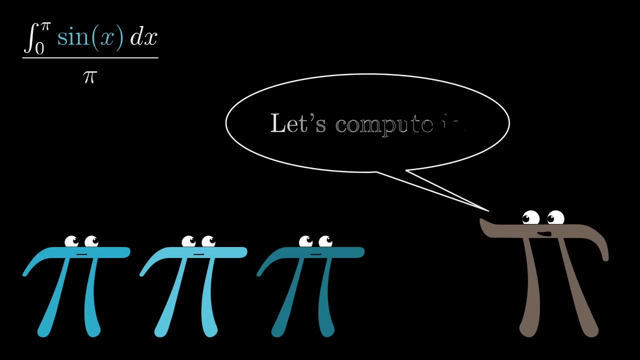 On an intuitive level and just thinking in terms of units, that feels pretty reasonable, doesn't it? Area divided by width, Width gives you an average height. So with this expression in hand, let's actually solve it. As we saw last video, to compute an integral, you need to find an antiderivative of the. 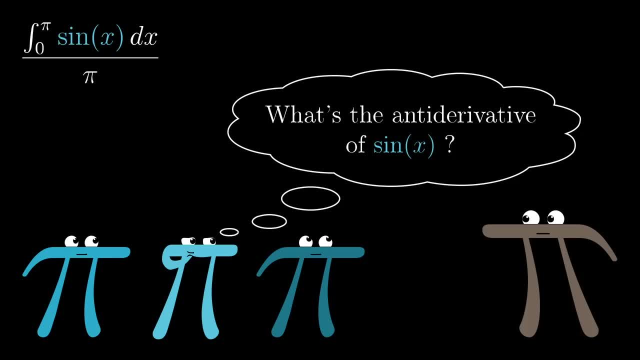 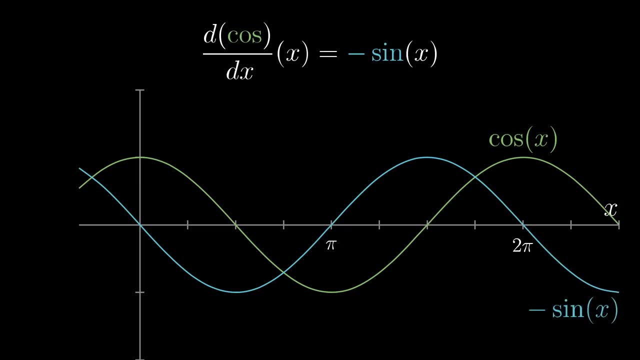 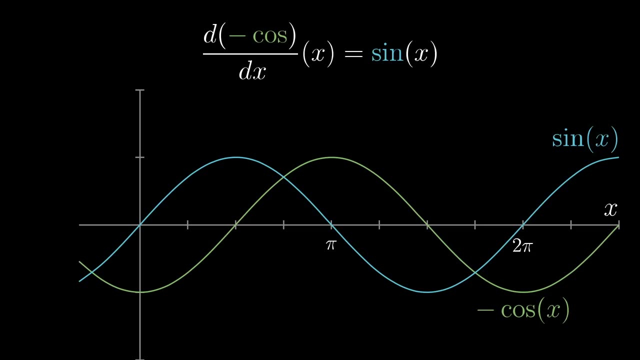 function inside the integral, some other function whose derivative is sine of x. And if you're comfortable with derivatives of trig functions, you know that the derivative of cosine is negative sine. So if you just negate that negative cosine is the function, we want the antiderivative. 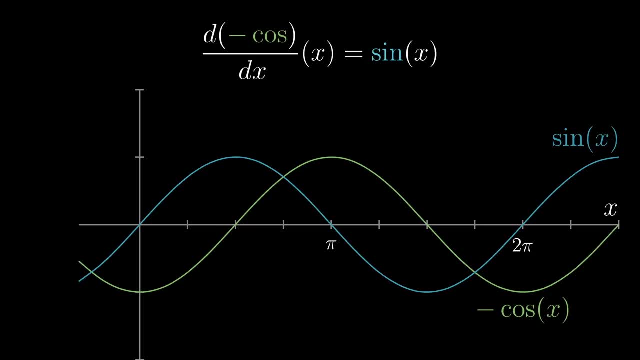 of sine. And to gut check yourself on that, look at this graph of negative cosine: At 0, the slope is 0. And then it increases up to some maximum slope at pi, halves and then goes back down to 0 at pi. 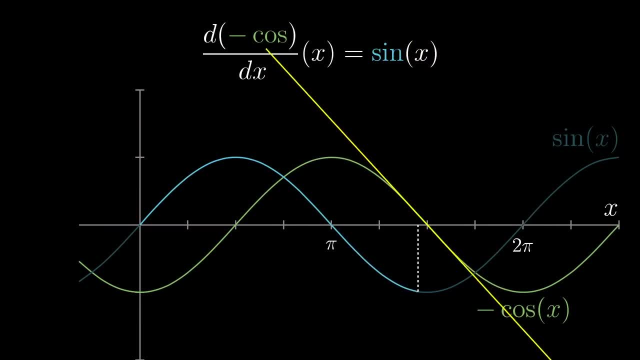 And in general, its slope does indeed seem to match the height of the sine graph at every point. So what do we have to do to evaluate the integral of sine between 0 and pi? Well, We evaluate this antiderivative At the upper bound. 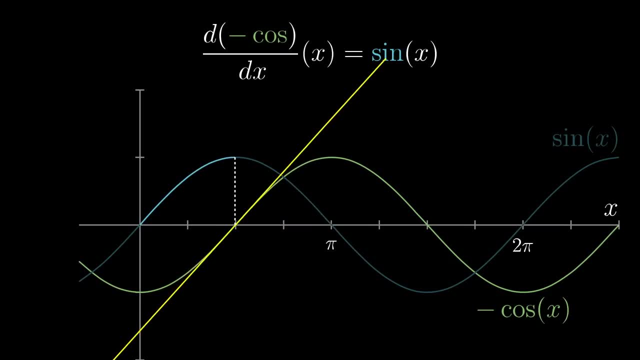 And then it increases up to some maximum slope at pi, halves and then goes back down to 0 at pi, And in general its slope does indeed seem to match the height of the sine graph at every point. So what do we have to do to evaluate the integral of sine between 0 and pi? 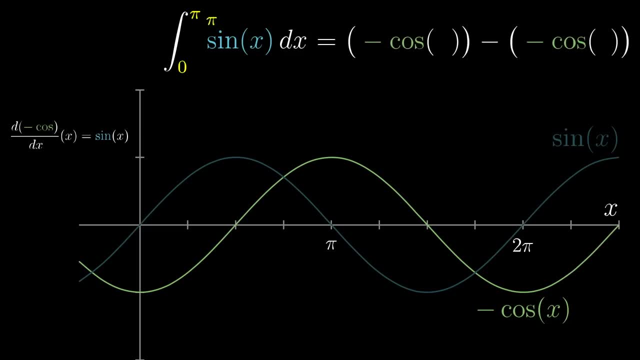 Well, We have to evaluate this antiderivative at the upper bound and subtract off its value at the lower bound. More visually, that is the difference in the height of this negative cosine graph above pi and its height at 0.. And as you can see, that change in height is exactly 2.. 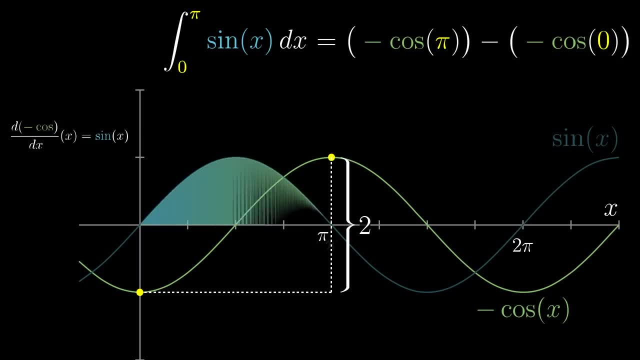 That's kind of interesting, isn't it, That the area under this sine graph turns out to be exactly 2.. So the answer to our average height problem, This integral divided by the width of the region, evidently turns out to be 2 divided. 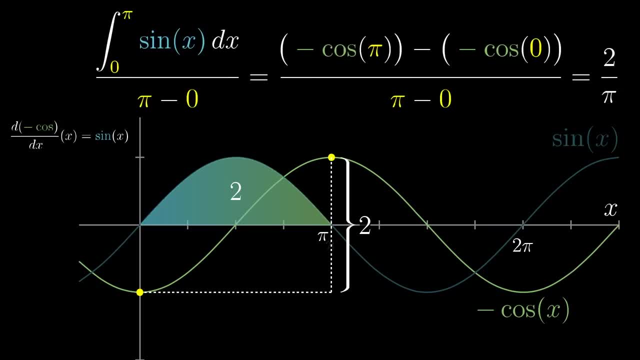 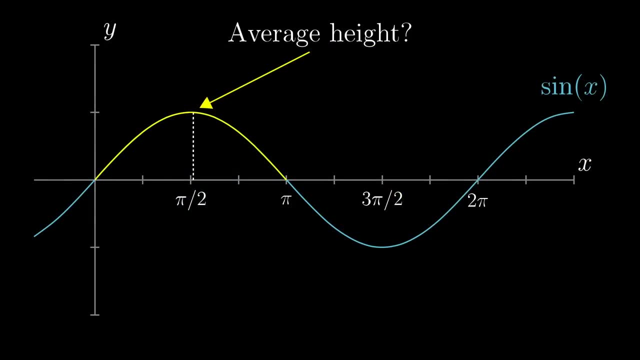 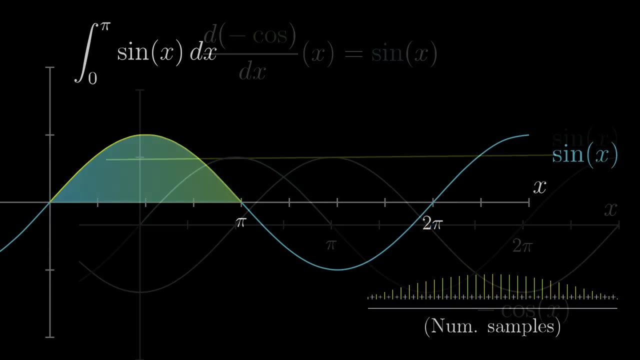 by pi, which is around 0.64.. I promised at the start that this question of finding the average of a function offers an alternate perspective on why integrals and derivatives are inverses of each other, why the area under one graph has anything to do with the slope of another graph. Notice how finding this average value 2 divided by pi came down to 0.. And that's exactly what we have to do to find the average of a function. Notice how finding this average value 2 divided by pi came down to 0.. 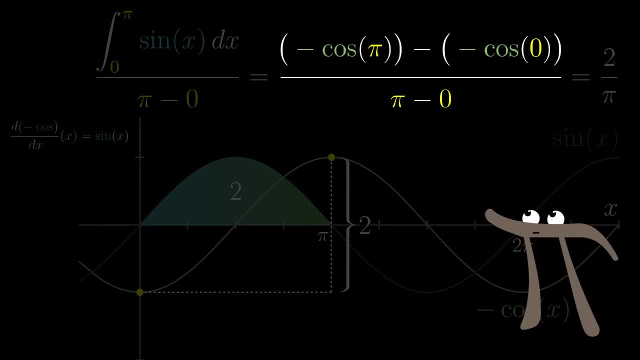 And that's exactly what we have to do: to find the average of a function où I've been looking at the change in the antiderivative Num4g5-cosx Conclusion And notice why this average value would represent the need for a new feature name, which is: 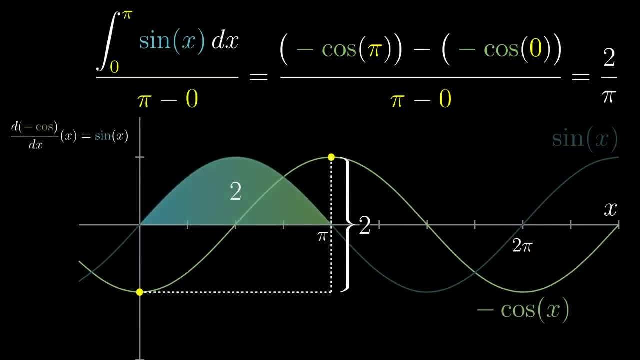 always in the range of the client in the beginning. Another way to think about that fraction is as the rise over the one, with a slope between the point of the antiderivative produced in the graph below 0, and the point of the graph above pi. 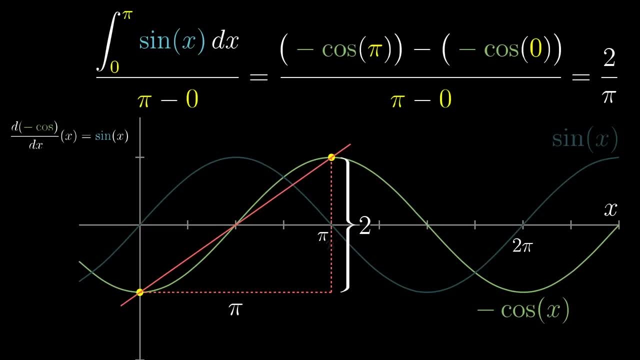 And why it makes sense that the number of originals that the gradient mangles from represents the Ads of x with that region And come to that end. you could also be asking yourself: why did you ever still have to think about that variable? Here we see Nurse d1. 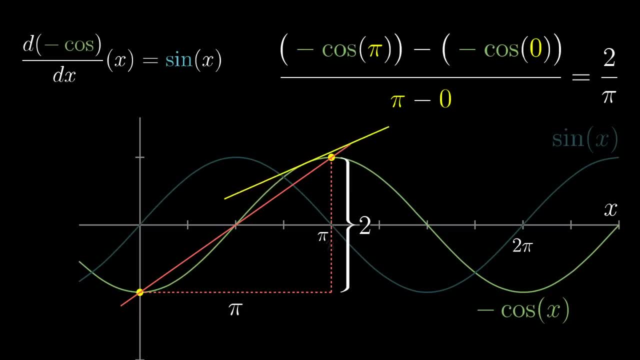 definition. sine of x is the derivative of this antiderivative graph. It gives us the slope of negative cosine at every point. So another way to think about the average value of sine of x is as the average slope over all tangent lines here between zero and pi. 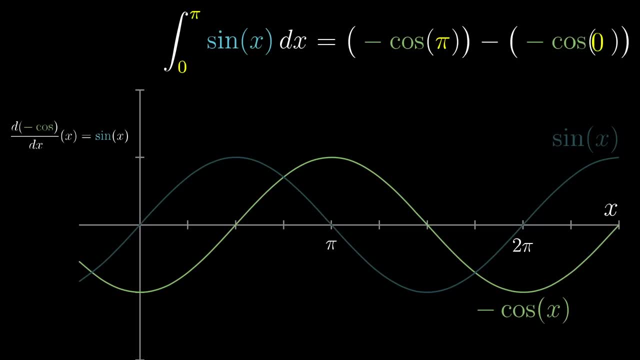 And subtract off its value at the lower bound. More visually, that is the difference in the height of this negative cosine graph above pi and its height at 0. And as you can see, that change in height is exactly 2.. That's kind of interesting, isn't it, that the area under this sine graph turns out to 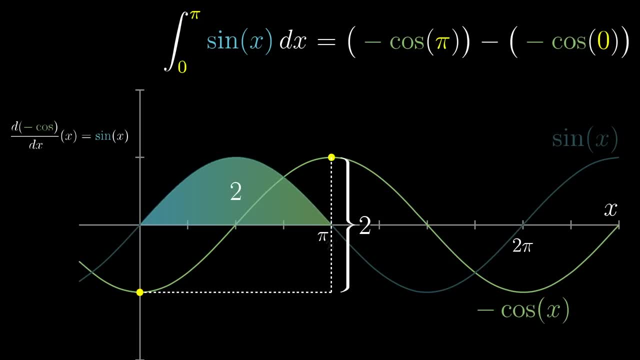 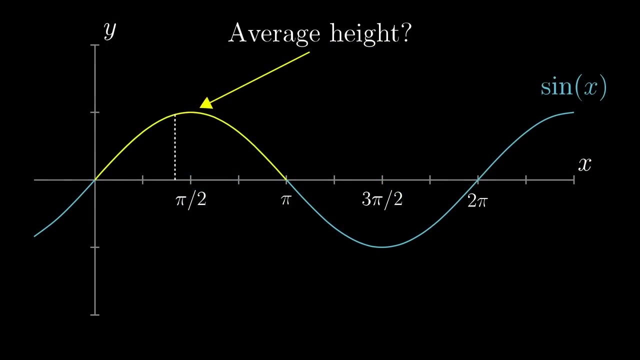 be exactly 2?. So the answer to our average height problem, this integral divided by the width of the region, Evidently turns out to be 2 divided by pi, Which is around 0.64.. I promised at the start that this question of finding the average of a function offers. 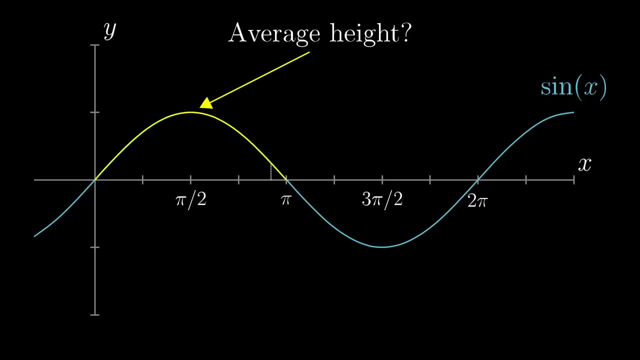 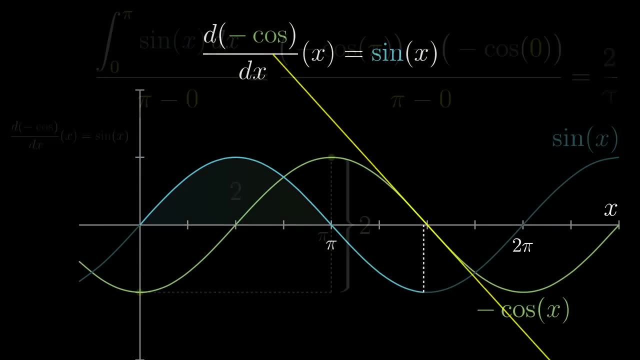 an alternate perspective on why integrals and derivatives are inverses of each other, Why the area under one graph has anything to do with the slope of another graph. Notice how finding this average value, 2 divided by pi, came down to looking at the change in. 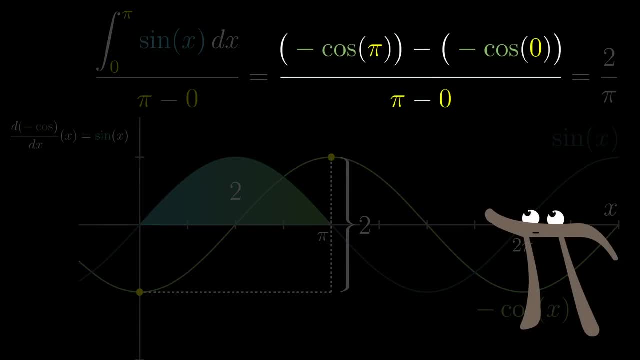 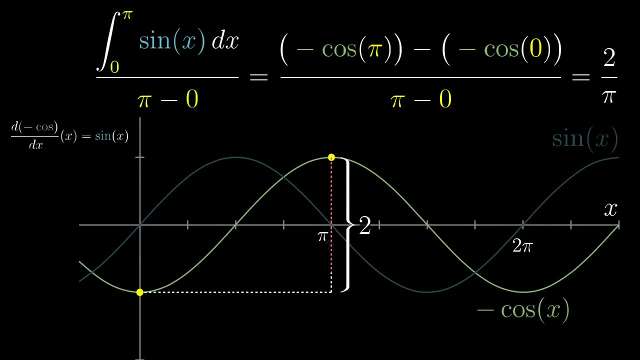 the antiderivative negative cosine, That is the antiderivative negative cosine x over the input range divided by the length of that range. And another way to think about that fraction is as the rise over run slope between the 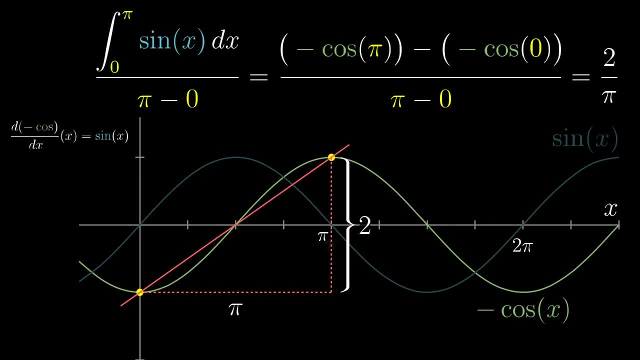 point of the antiderivative graph below 0, and the point of that graph above pi. And now think about why it might make sense that this slope would represent an average value of sine of x on that region. By definition, sine of x is the derivative of this antiderivative. 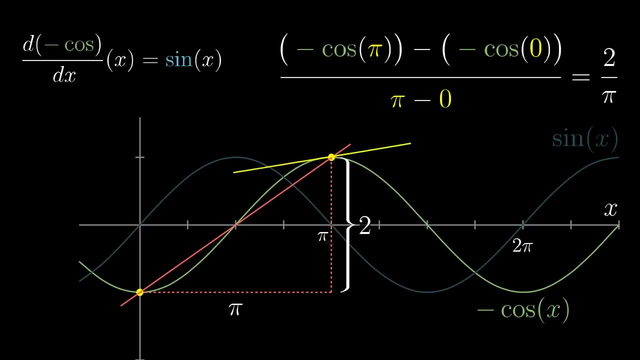 It gives us the slope of negative cosine at every point. So another way to think about the average value of sine of x is as the average slope over all tangent lines here between 0 and pi. And when you view things like that doesn't it make a lot of sense that the average slope 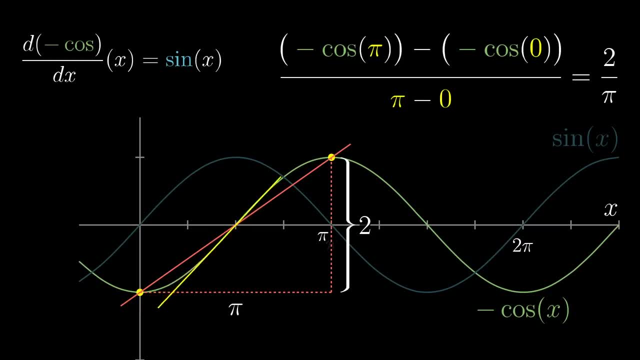 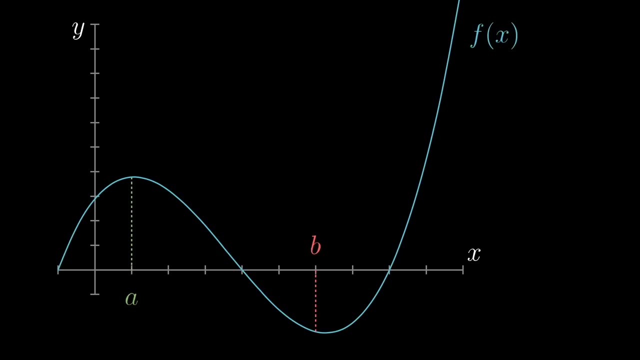 of a graph over all of its points in a certain range should equal the total slope between the start and end points. Yes, Yes, Yes. So to suggest this idea. it helps to think about what it looks like for a general function, For any function f, if you want to find its average value on some interval, say: 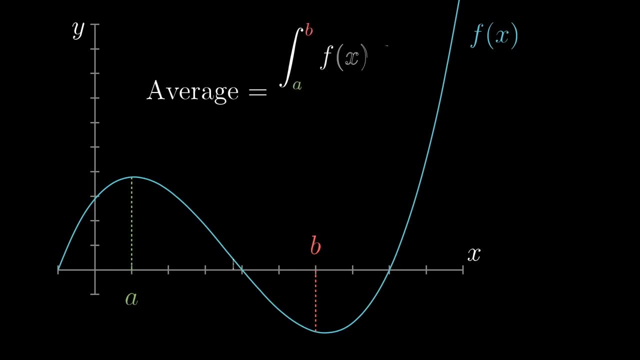 between a and b. what you do is take the integral of f on that interval divided by the width of that interval. You can think of this as the area under the graph divided by its width or, more accurately, it is the signed area of that graph, since any area below the x-axis is counted as negative. 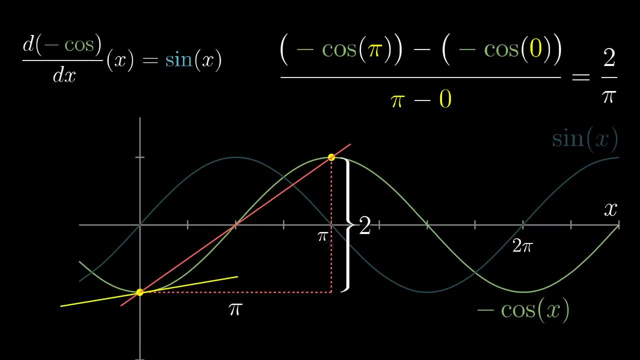 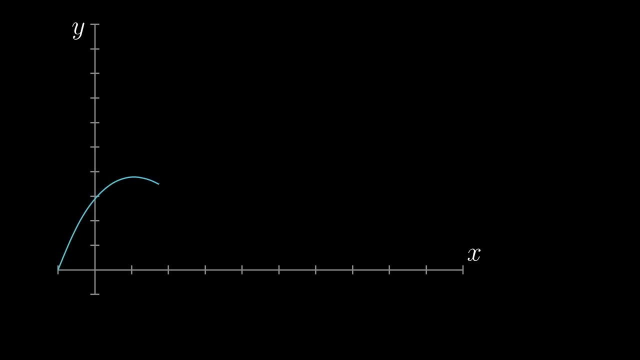 And when you view things like that, doesn't it make a lot of sense that the average slope of a graph over all of its points in a certain range should equal the total slope between the start and end points. To digest this idea, it helps to think about what it looks like for a general function. 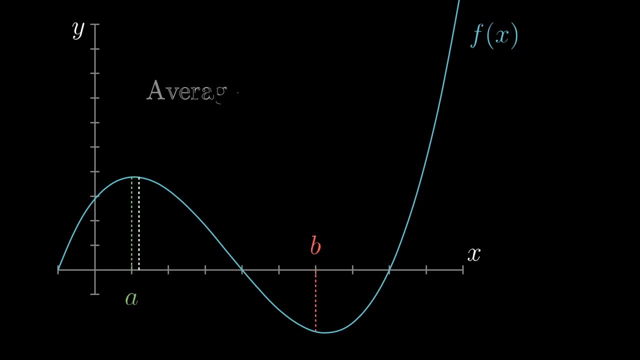 For any function, f, if you want to find its average value on some interval, say between a and b, what you do is take the integral of f on that interval divided by the width of that interval b-a. You can think of this as the area under the graph divided. 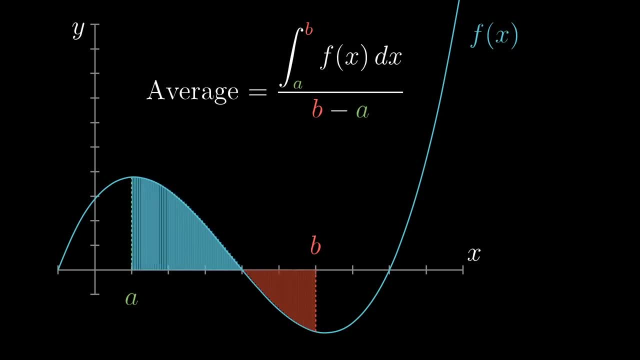 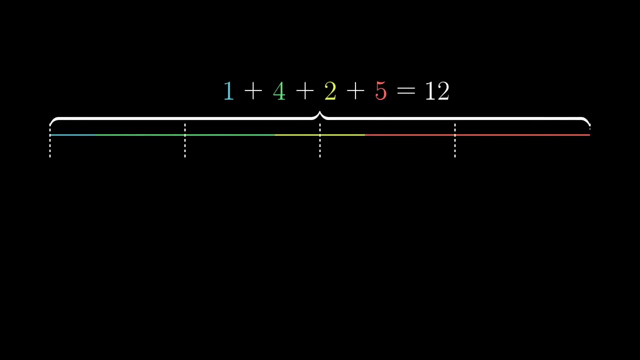 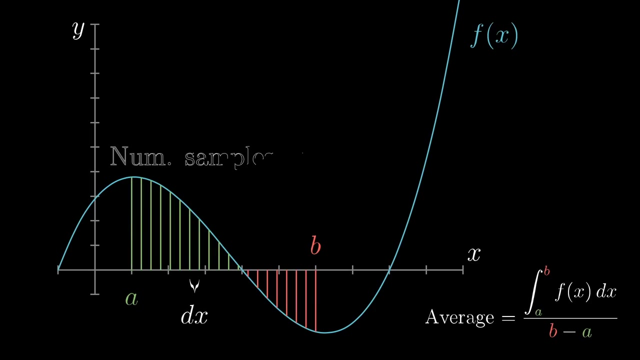 by its width, Or more accurately, it is the C, And it's worth taking a moment to remember what this area has to do with the usual notion of a finite average, where you add up many numbers and divide by how many there are. When you take some sample of points spaced out by dx, the number of samples is about: 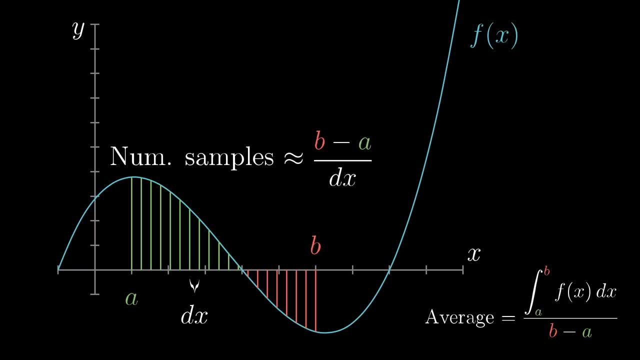 equal to the length of the interval divided by dx. So if you add up the values of f at each sample and divide by the total number of samples, it's the same as adding up the product f and dividing by the width of the entire interval. 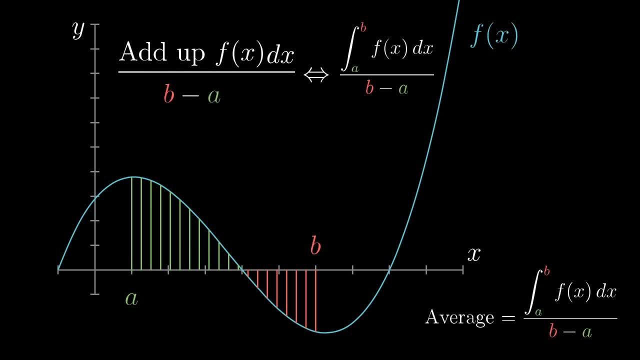 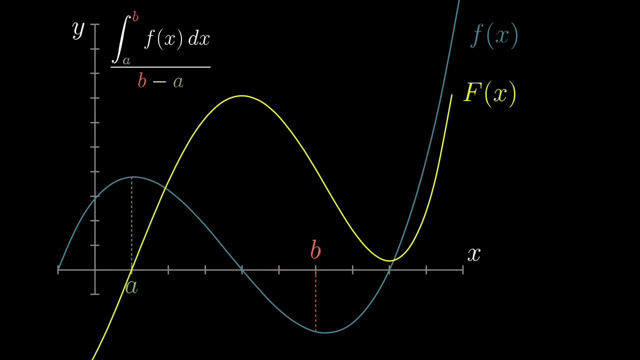 The only difference between that and the integral is that the integral asks what happens as dx approaches zero. but that just corresponds with samples of more and more points that approximate the true average increasingly well. For any integral evaluating, it comes down to finding an antiderivative of f. 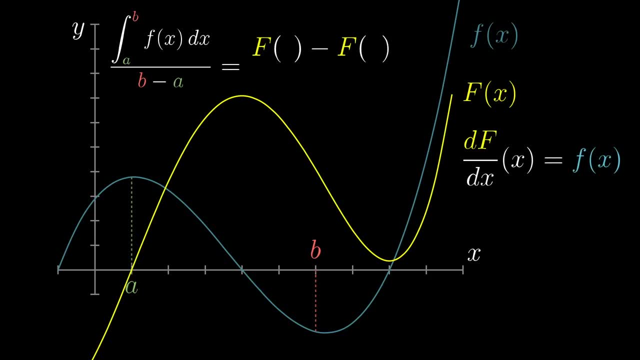 commonly denoted capital F. What we want is the change to this antiderivative between a and b capital F, which you can think of as the change in height of this graph between the two bounds. I've conveniently chosen an antiderivative that passes through zero at the lower bound. 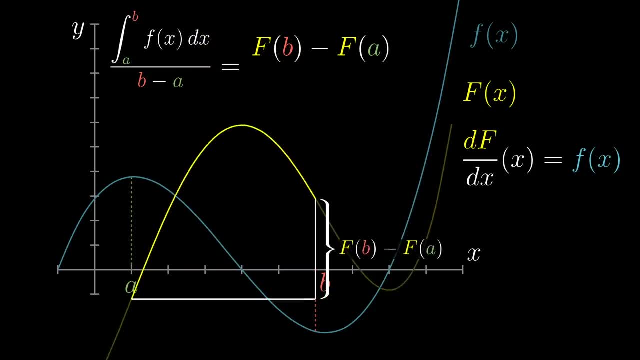 here. but keep in mind you can freely shift this up and down, adding whatever constant you want to it. It would still be a valid antiderivative. So the solution to the average problem is the change in the height of this new graph, divided by the change to the x value between a and b, In other words, 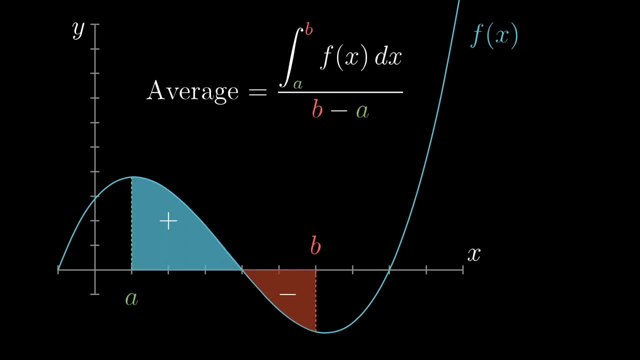 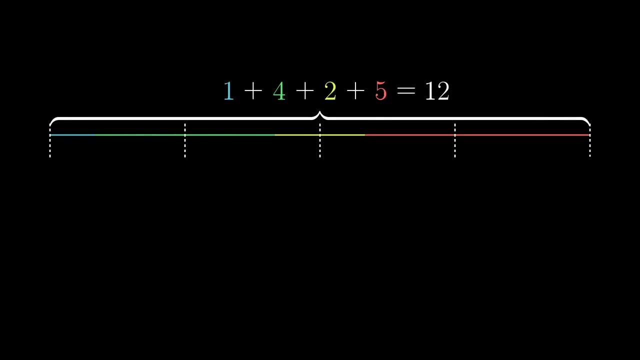 And it's worth taking a moment to remember what this area has to do with the usual notion of a finite average, where you add up many numbers and divide by how many there are. When you take some sample of points spaced out by dx, the number of samples is about: 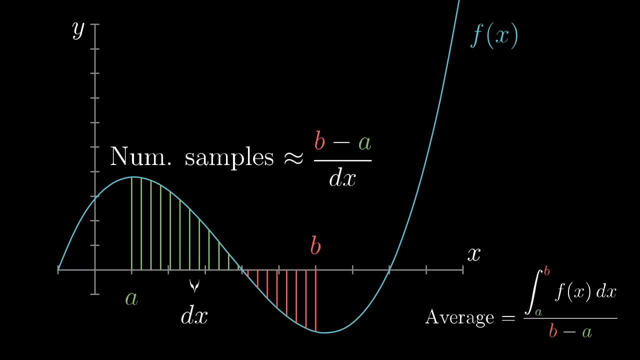 equal to the length of the interval divided by dx. So if you add up the values of f at each sample and divide by the total number of samples, it's the same as adding up the product f times dx and dividing by the. 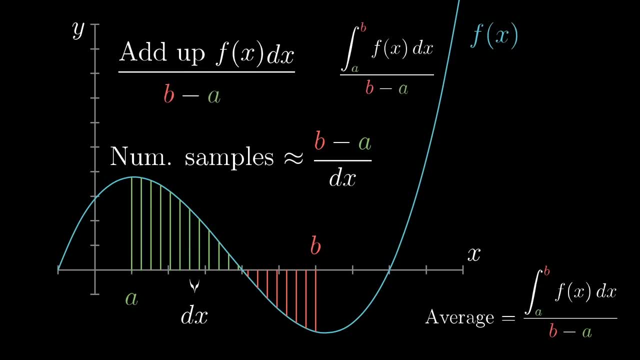 width of the entire interval. The only difference between that and the integral is that the integral asks what happens as dx approaches zero. but that just corresponds with samples of more and more points that approximate the true average increasingly well. For any integral evaluating it comes down to finding an antiderivative of f. commonly 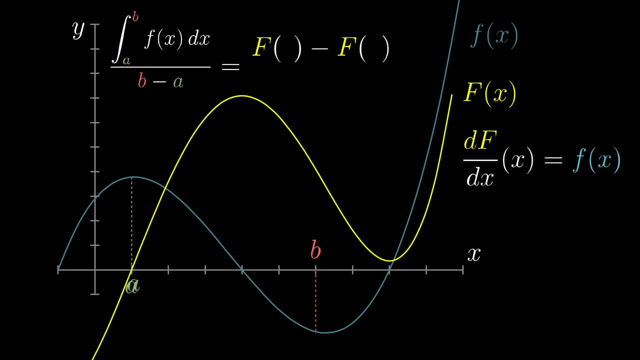 denoted kappa. What we want is the change to this antiderivative between a and b, capital F of b minus capital F of a, which you can think of as the change in height of this new graph between the two bounds. I've conveniently chosen an antiderivative that passes through zero at the lower bound. 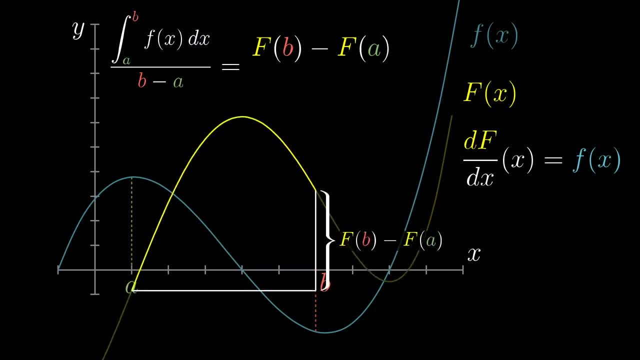 here. but keep in mind, you can freely shift this up and down, adding whatever constant you want to it, and it would still be a valid antiderivative. So the solution to the average problem is the change in the height of this new graph. 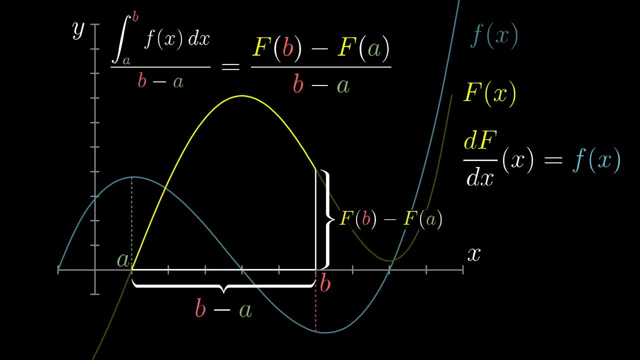 divided by the change to the x-value between a and b. In other words, it is the slope of the antiderivative graph between the two endpoints. And again, when you stop to think about it, that should make a lot of sense, because little. 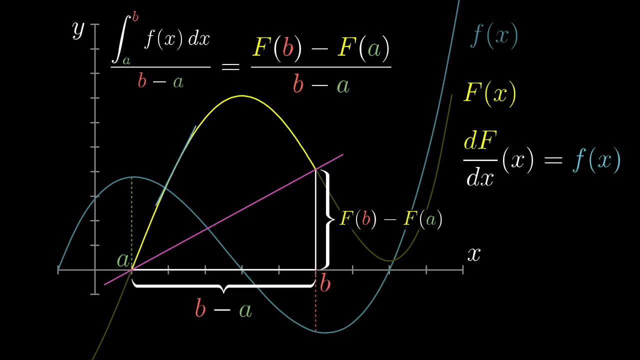 f gives us the slope of the tangent line to this graph at each point. After all, it is by definition the derivative of the antiderivative. So the solution to the average problem is the change in the height of this new graph, divided by the change to the x-value between a and b.